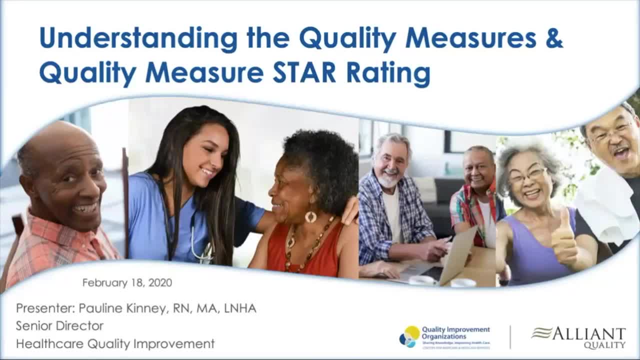 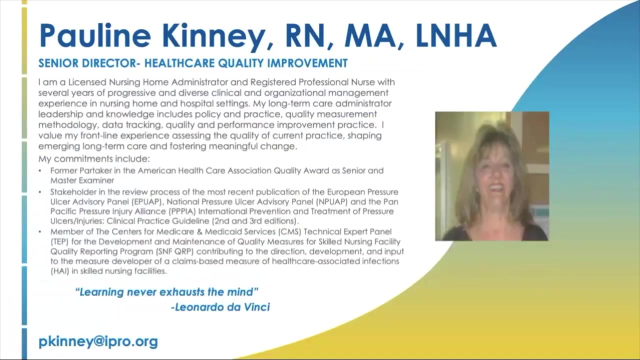 and to use this time to share some interesting information about the quality measures. I would like to start the program by sharing a bit about myself and my transition into quality improvement. I started my career in the acute care industry as an emergency room nurse. After many years in the ER, a light bulb went off. I began to focus more on the condition of 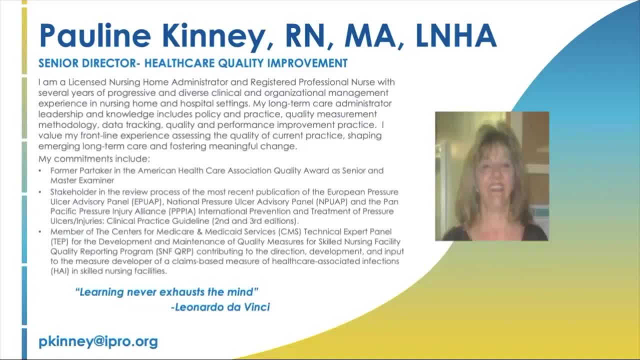 the residents coming to the ER and the short amount of time dedicated to addressing their needs. I found myself in the ER for a long time and I've been doing this for a long time. I've been wondering about the residents' well-being after discharge. 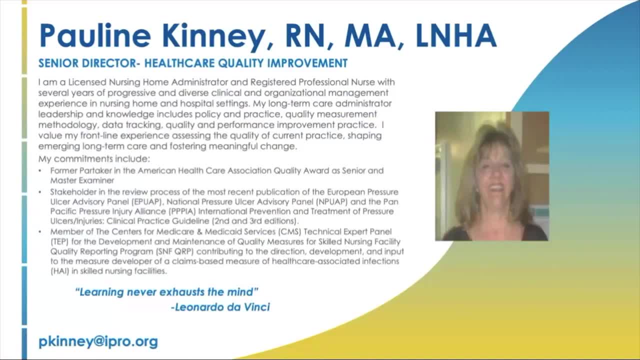 It was at this point that I decided maybe I should change course and use my knowledge and skill to address the care of the elderly. So I transitioned to long-term care as a nursing home administrator and I am happy to say that I did make positive change in the facilities that 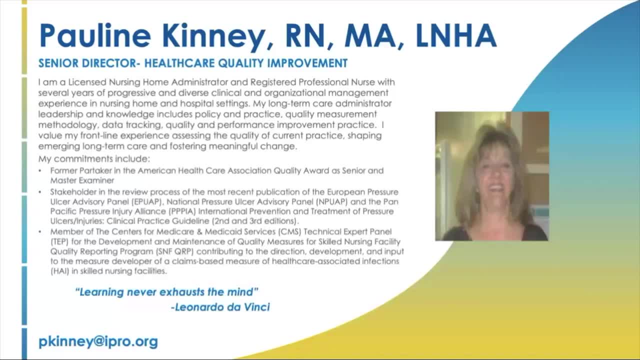 I worked in by building and guiding a team of staff through sustainable resident quality and safety strategies and practices. A second light bulb went off and I reached a point where I thought it may be time to expand my knowledge and passion for quality to a wider 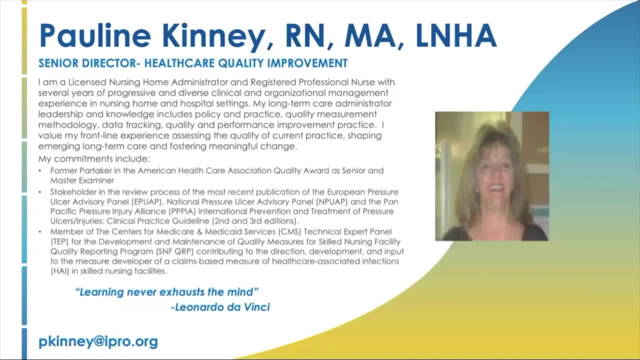 audience. It was at that point that I joined the QIO. It was a perfect opportunity. It was the onset of CMS's recognition of the quality improvement organization's quality improvement work in long-term care. That was 18 years ago, and in that time I have had the pleasure of leading a team of 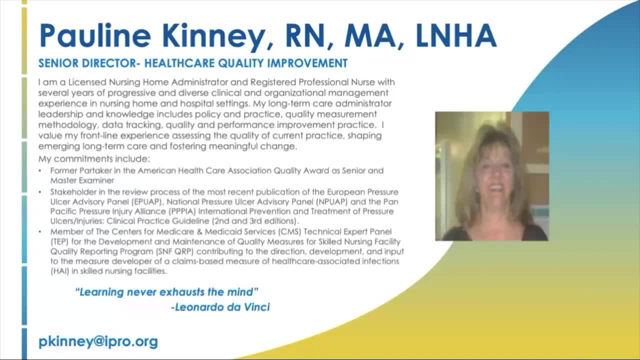 professionals and working with hundreds of statewide nursing homes on their quality improvement programs, So I'm happy to be with you today. Together, we can begin to think about what changes we would like to make in our individual facilities and how we can use the quality measures as the starting point to change. 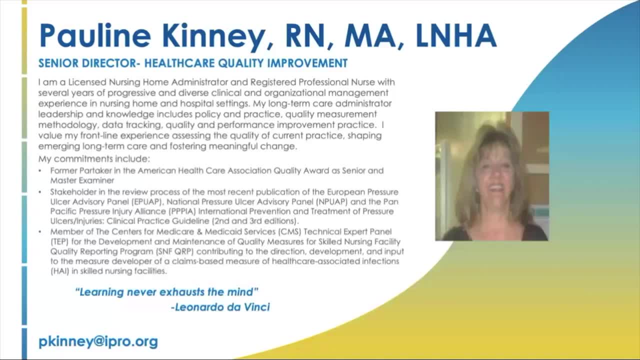 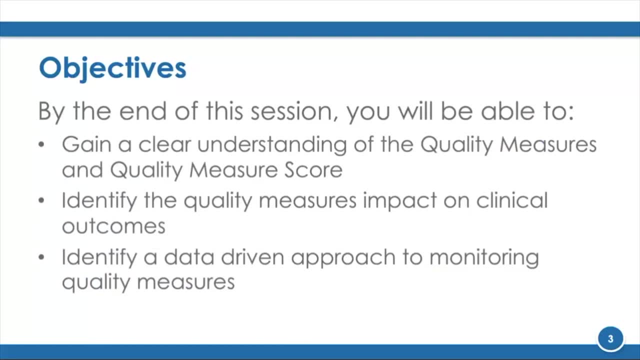 The purpose of today's presentation is to introduce, or, for some of you, to reintroduce, the quality measures, the quality measure score and its impact on the overall star quality measure rating and overall five-star rating. As we work throughout the Nursing Home Quality Care Collaborative, we will take a deeper dive into the total quality measure. 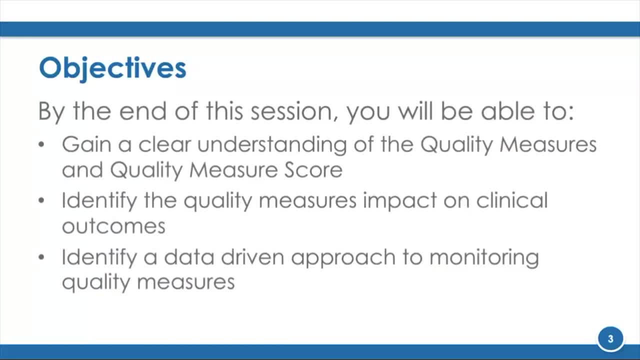 score- QM star rating- and we will highlight tools for the quality measure score. and we will highlight tools for the QM star rating and overall five-star rating. As we work through the QM star rating, we will highlight tools to self-calculate and monitor your individual. 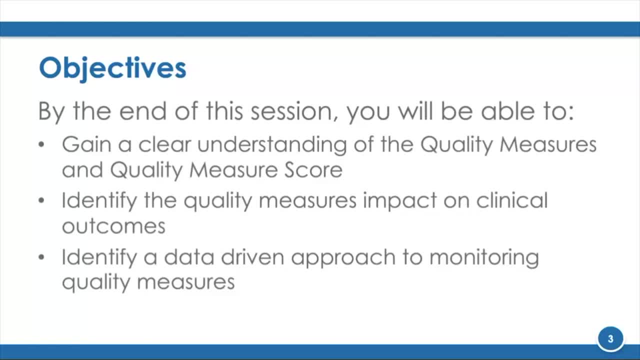 nursing home score, thus working to identify and address opportunities for improvement. I will guide you through the presentation today and by the end of the session. the aim is that you will have gained a clear understanding of the quality measures and quality measure score, identified how the quality measures impact clinical outcomes and identified a 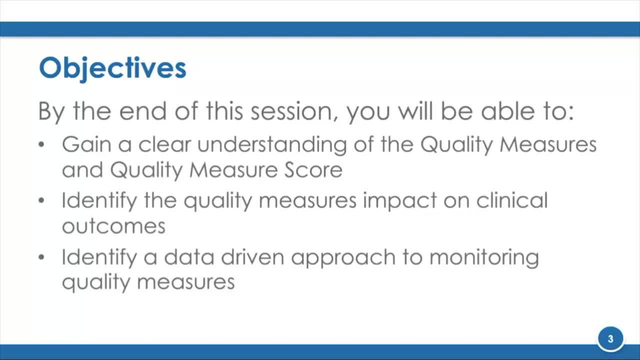 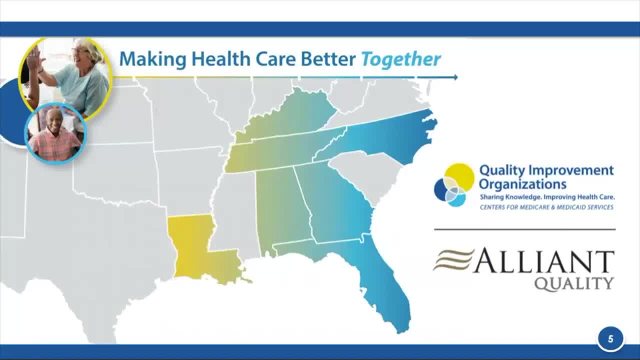 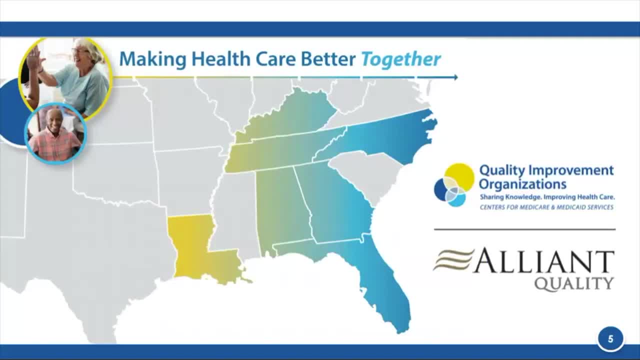 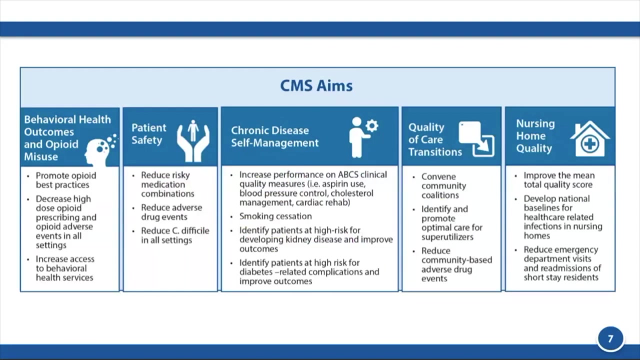 Kentucky, Louisiana, North Carolina and Tennessee. focusing on quality, Alliant Quality has worked on quality improvement with providers, clinicians and beneficiaries across the Southeast to collaborate to make healthcare better for almost 50 years. You can see from this slide the several important and focused CMS aims. 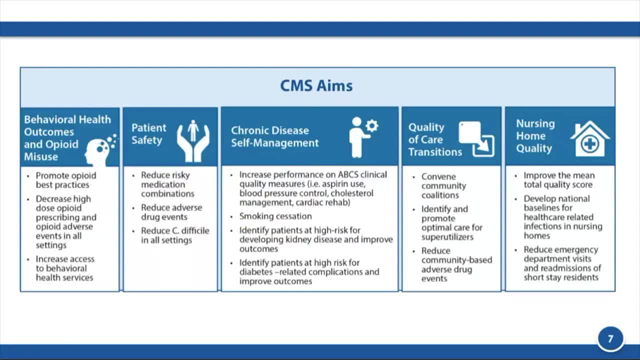 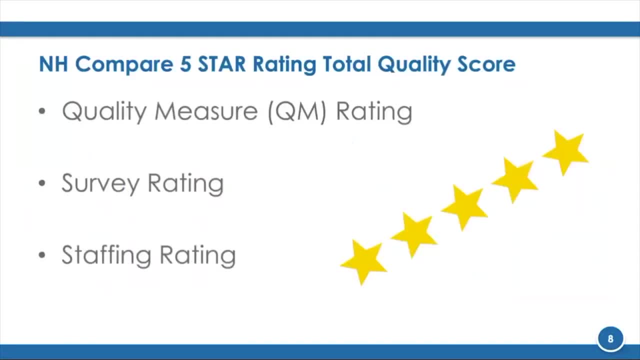 Today's presentation will focus on a component of the last aim, or nursing home quality. Recognizing the multidimensional nature of nursing home quality, the overall five-star rating total quality score posted to Nursing Home Compare displays quality score ranking from three areas: quality measure ranking, survey ranking and staffing ranking. 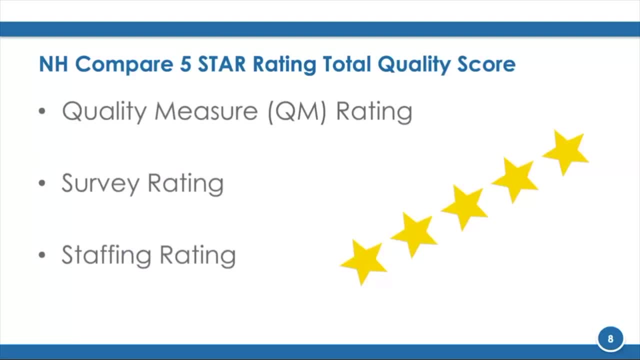 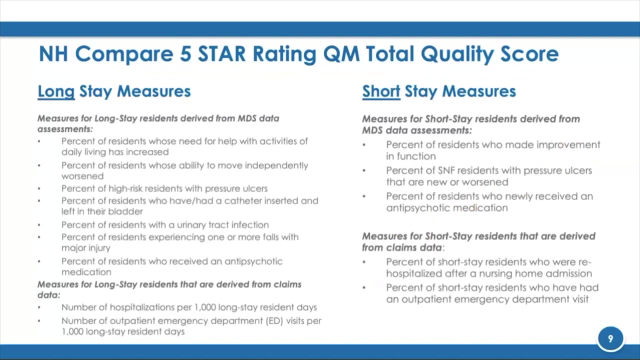 For the purpose of this presentation, we'll be focused on understanding and improving the quality measures, their total quality score and corresponding quality scores. Not all quality measures reported on Nursing Home Compare are included in the calculation of the quality measure, total quality score and star rating. 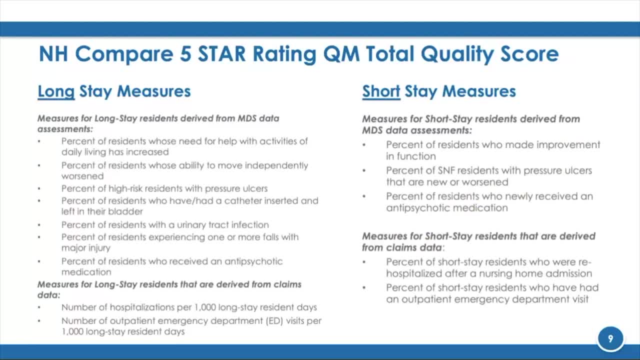 CMS utilizes a range of data sources to calculate quality measure score. The 15 long and short-stay measures listed on the slide are the measures that are most likely to impact the QM total quality score. So where do the quality measures come from? 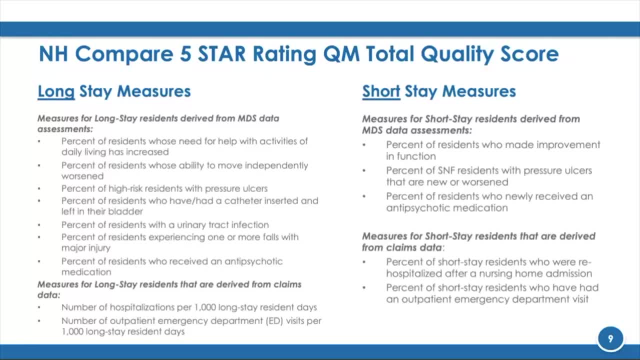 Well, the quality measures were developed using MDS clinical-based measure data and Medicare claims data submitted for Medicare fee-for-service residents. that describes the quality care provided in the nursing home. So you may ask: why these measures? Well, the 15 measures were selected for use in the nursing home. 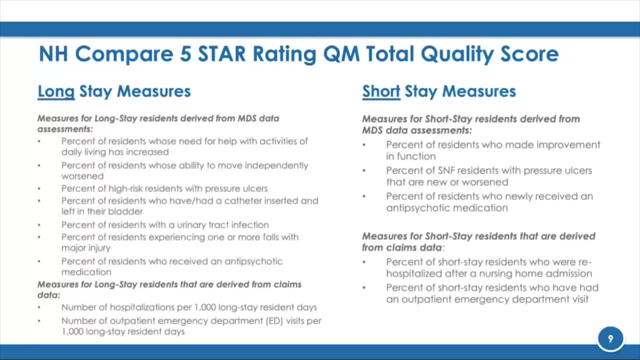 The 15 measures were selected for use in the nursing home. The 15 measures were selected for use in the rating system based on their importance and extent to which the nursing home's practice affects the measures. Data for the MDS-based quality measures and the claims-based measures are updated quarterly. 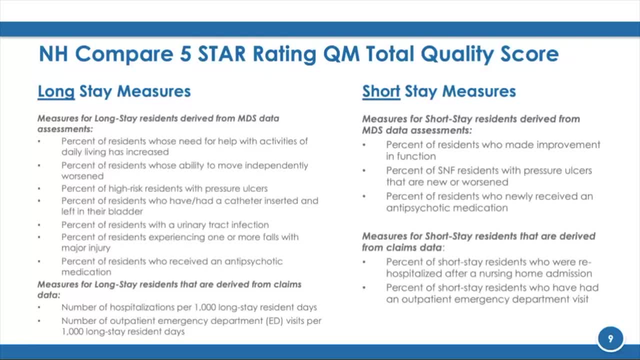 and the QM rating is updated at the same time. The updates typically occur in January, April, July and October at the time of the Nursing Home Compare website refresh. So as the quality measures are one-third of the total quality score component, you can: 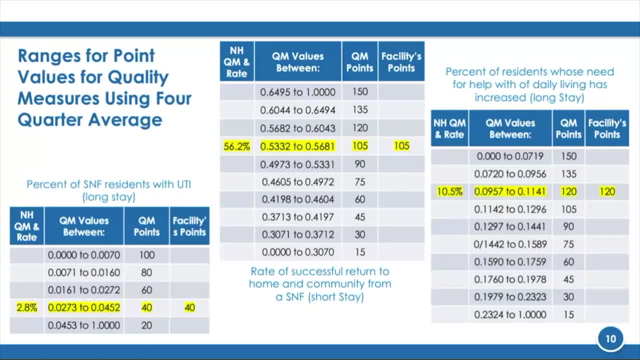 see how changes in the quality measures may affect the change the facility overall star rating. So you may be wondering where the long and short-stay pain quality measures are. Well, the pain measures have been removed from the Nursing Home Compare website and the five star quality rating system in October of 2019.. 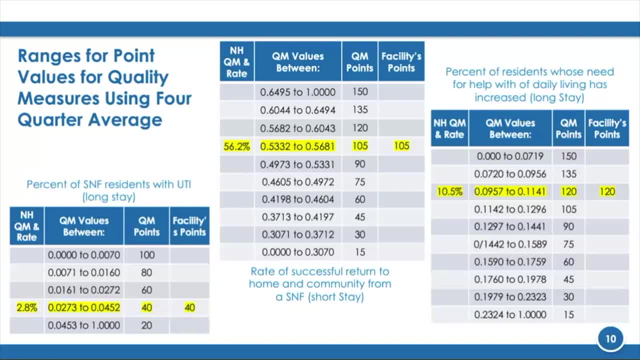 The information that I've seen from CMS pertaining to the removal of the pain measures, links to the federal initiative to reduce opioid utilization and the aim to prevent the potential scenario where the performance of the facility on the pain quality measure may inappropriately contribute to their decision to seek the administration's approval. 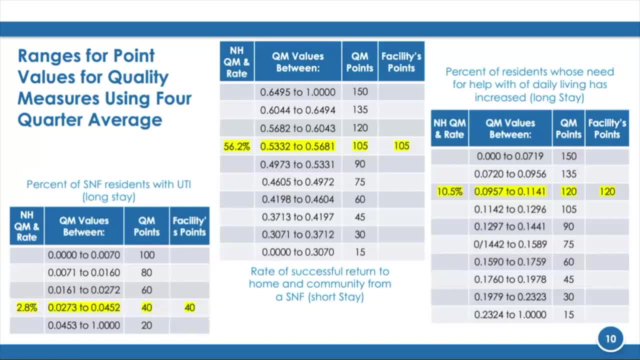 So the information that I've seen from CMS pertaining to the removal of the pain measure links to the federal initiative to reduce opioid utilization and the aim to prevent the potential scenario where the facility on the pain measure may inappropriately contribute to the decision to seek the administration of an opioid. 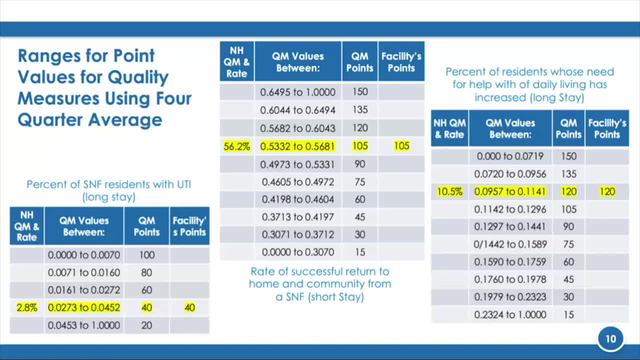 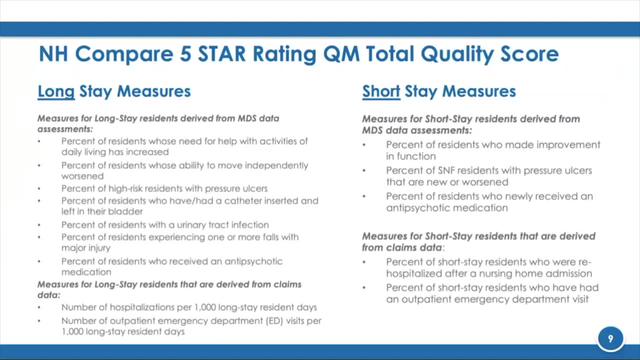 So you can see, the 15 measures are comprised of 10 clinical measures and five claims-based measures. The five claims-based measures are the long and short-stay readmission and emergency department visits and successful return to home or community and, as mentioned, there is no longer long. 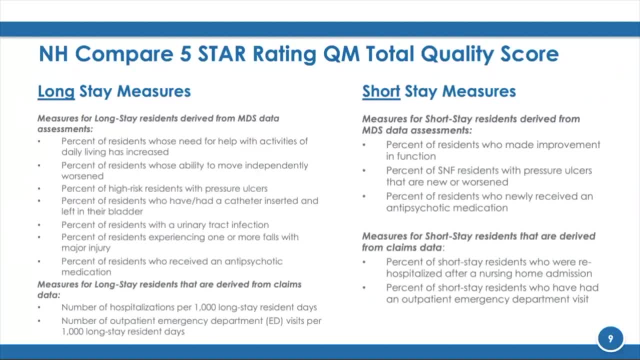 or short-stay pain quality measures. Remember, when comparing the long and short-stay measures: the long-stay measure is defined as residents who are in the nursing home for greater than 100 days and the short-stay measure is defined as residents who are in the nursing home for less than 100 days. 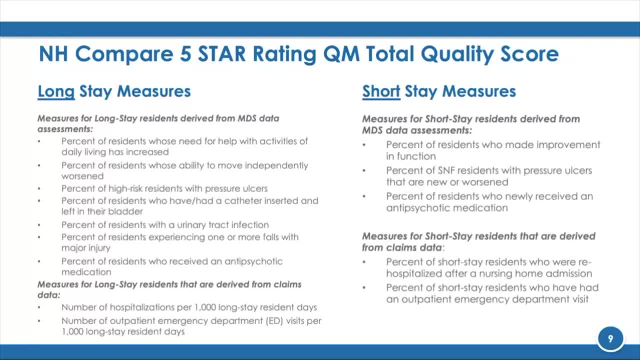 The slide is a bit busy, but you may find it useful to keep the list of the 15 measures close by for reference and review how they factor in your individual performance. And if you have any questions, please feel free to reach out to me at the call center. 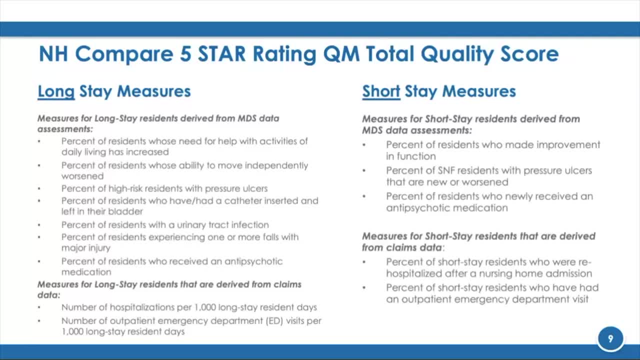 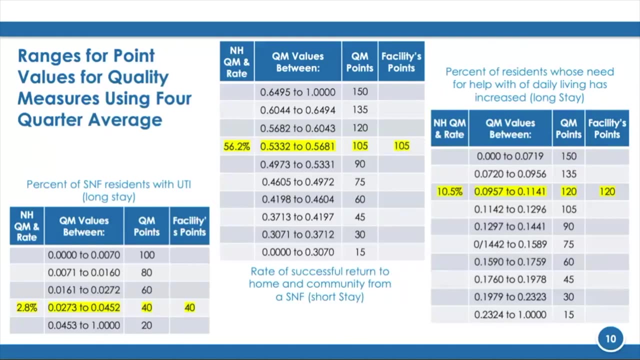 at the end of this webinar. Thank you very much. individual facilities, assessment of care practices and the QM score. now that we know the measures, let's look at where the point values come from and how they tie into the quality measure scores. again, a busy slide, but let's drill this. 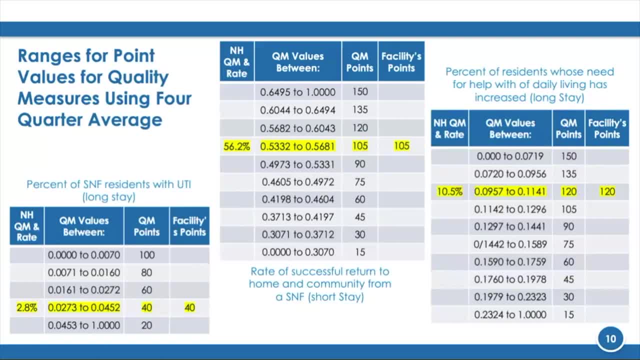 down a little bit. so when we look at the quality measures and their quality measure star rating, it is not only important to understand where the point values and the star designation comes from, but also what to do with the information to improve the quality measure score. so we've learned that CMS. 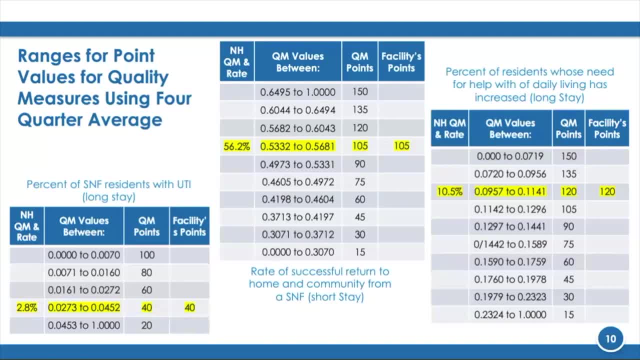 calculates the quality measure points and ratings based on the performance on a subset of 10 MDS based and five measures that are created using Medicare claims, and that the 15 measures were selected for use in the rating system based on their validity and reliability and to the extent which nursing home practice may affect the 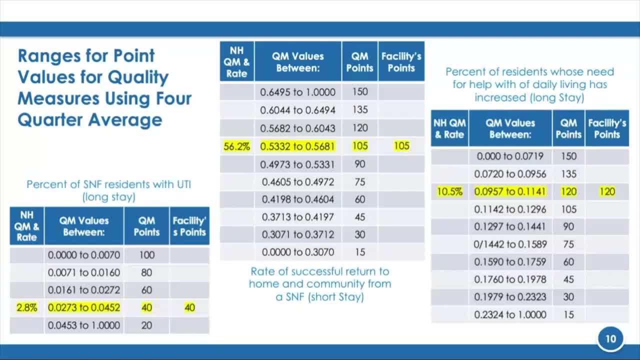 measures. so with that and moving on, two different sets of weights are used for assigning individual QM points. some measures have a maximum score of 150 points, while others have a maximum score of 100 points. the weight for each measure is determined based on the opportunity for. 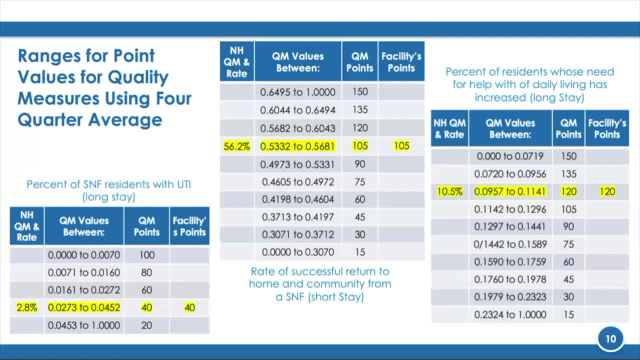 the nursing home to improve the measure and the clinical significance of the measure, based on expert feedback. again looking at the 15 quality measures: for measures that have a maximum of 150 points, the points are factored in 10 equal sections or deciles. the QM that have the 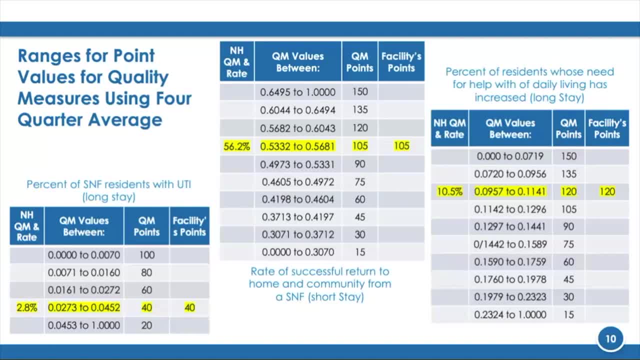 potential of 150 points include the long-stay ADL worsening, long-stay antipsychotic medication, long-stay mobility decline, the two claims-based long-stay measures, the short-stay functional improvement and the three claims-based short-stay measures For the measures that have a maximum of 100. 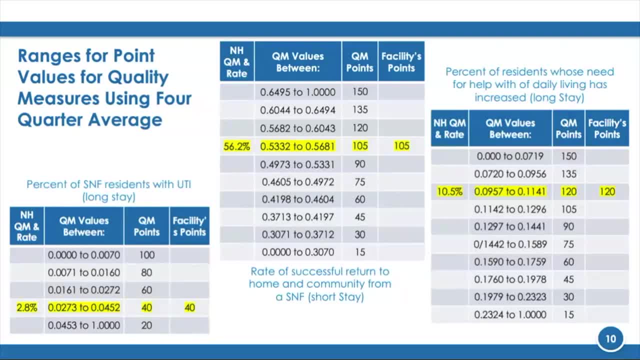 points. the points are factored in five equal sections or quintiles. The QMs that have the potential of 100 points include: long-stay pressure ulcer. long-stay catheter, long-stay UTI, long-stay falls, short-stay pressure ulcer and short-stay. 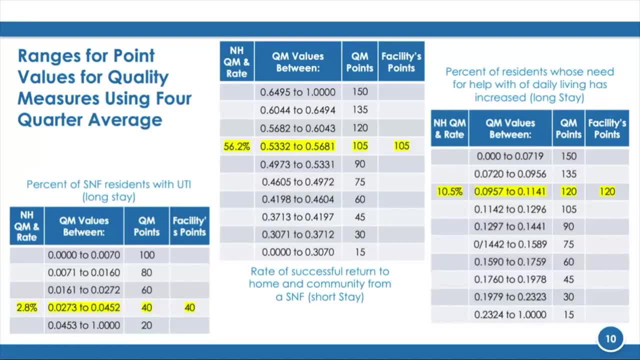 antipsychotic medication use. For all of the measures, points are calculated based on performance relative to the national distribution of the measure or the QM rate. Having a greater number of points corresponds to better performance. More points are rewarded for having a lower. 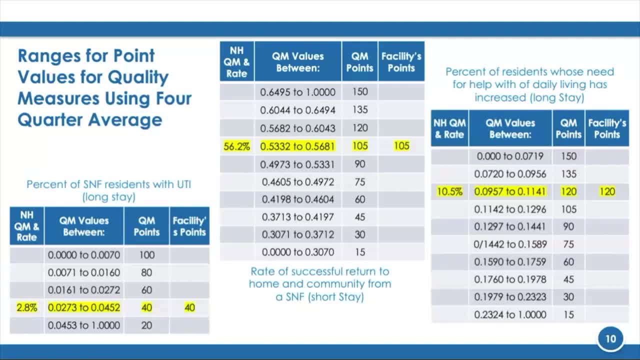 QM rate, except the functional improvement and successful home community discharge, whereby higher rates correspond to better performance. Next slide. So you may be asking: where can I see the points that are awarded to the facility for each of the QMs? I do not believe the point value is available to you, but what is available to you, and the point of this slide, is that you have the ability to calculate your own points and thus establish areas that are in need of improvement and potential points needed to get you to a heightened star rating. 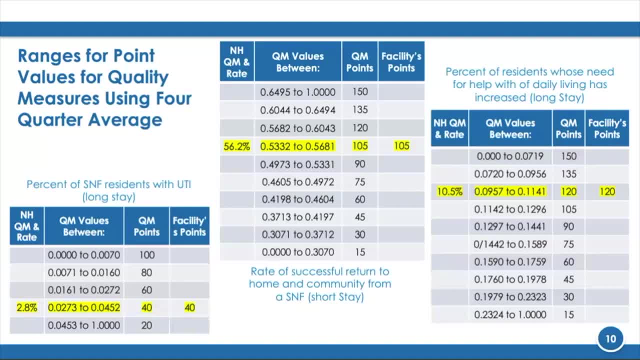 So I will share a resource with you in the next few slides where you can get this information. But let us look at this example. This nursing home has a 2.8% QM rating for the long-stay UTI quality measure. 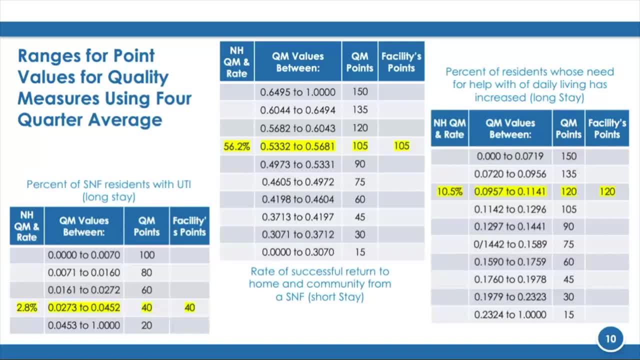 You can see that on the left side of your slide. Looking at the QM cut point values, you can see that it falls in the 40-point category. Therefore, the facility has 40 points awarded for this measure. Then we look at the successful return to the community and the rate of 56.2%, that's, the center awards 105 points, and so on. 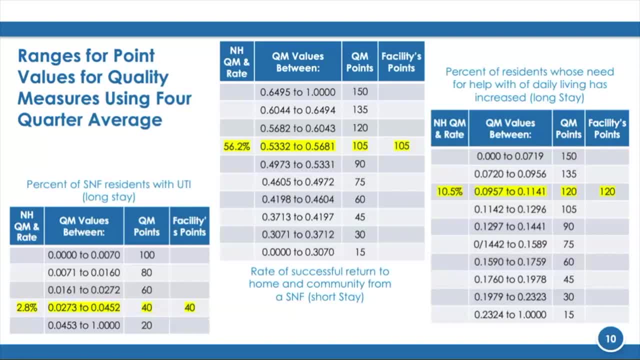 The points are summed across all of the measures and totaled to create a QM score. This slide provides you with a sample, but the official ranges for point values for the 15 quality measures is available to you in Table 2 of the October 2019 CMS Technical User's Guide. 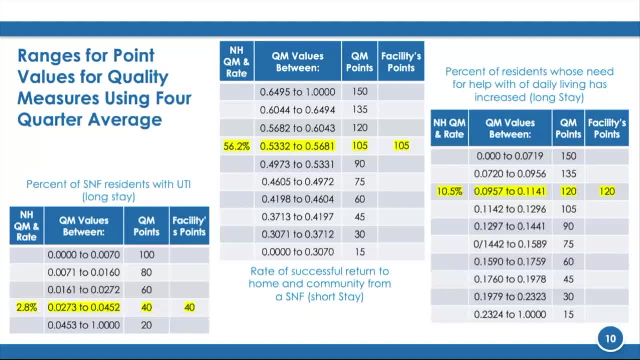 I've seen an electronic point calculator tool similar to that of the composite measure score calculator for those of you who remember the composite measure in previous scopes of work. However, I believe there may be some updating to it so we can keep you posted on the tool. 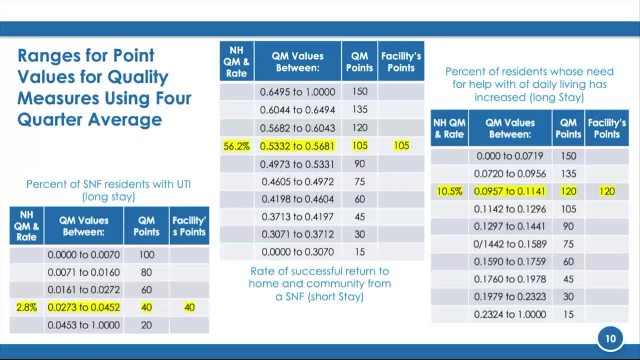 As it comes available For the recap. we know the 15 quality measures that are used to assess the quality in our facilities and we know how our facilities are rewarded- points for the quality measures. Now let's see how the points are converted to an overall quality measure star rating. 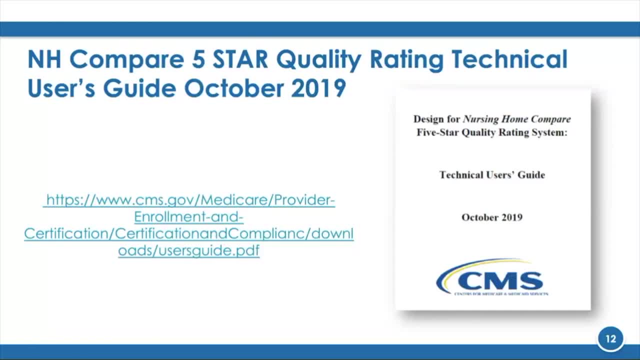 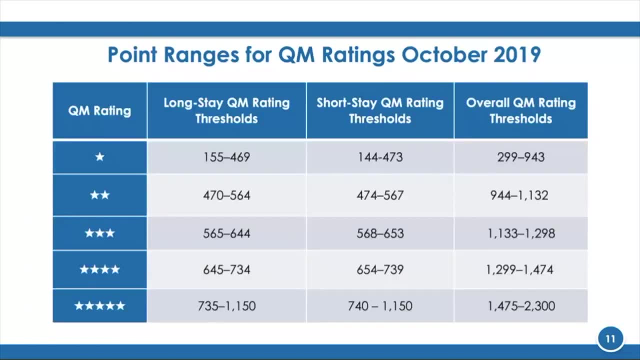 Most nursing homes will have three QM ratings: a long-stay QM threshold, a short-stay QM threshold and a short-stay QM threshold. Points are summed across. all the long and short-stay end facilities received an overall QM rating. 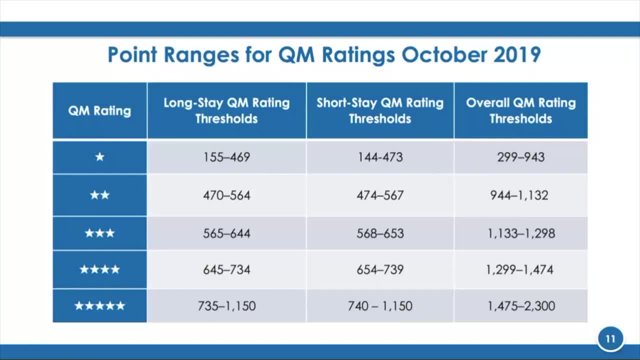 For nursing homes that have only long-stay or short-stay QMs, the overall QM rating is equal to their long or short-stay QM rating. So, looking at this chart, you can see how the cut points determine the nursing homes. 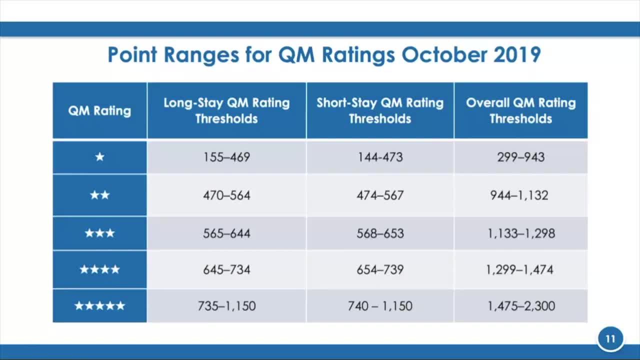 overall QM star rating. So if you sum the long and the short-stay measures, it equals an overall QM rating of a thousand points. By looking at the threshold chart, you can see that the point value falls within the two-star overall QM rating threshold. 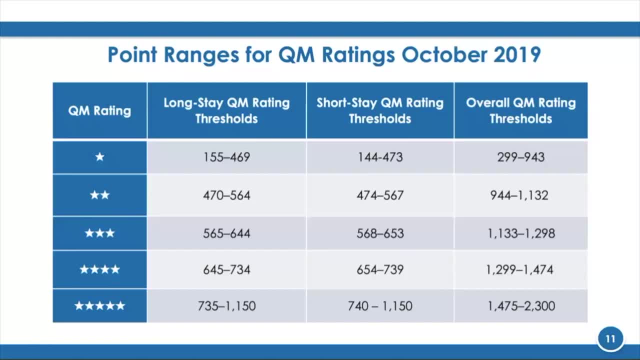 So this is the rating that your facility will have and will be posted on the tool. Thank you, And now I'm going to go over what we've listed to nursing home. compare Survey and staffing domains also have calculated cut points. But remember, for the purpose of this presentation we are only looking at the QMs and their ranking. 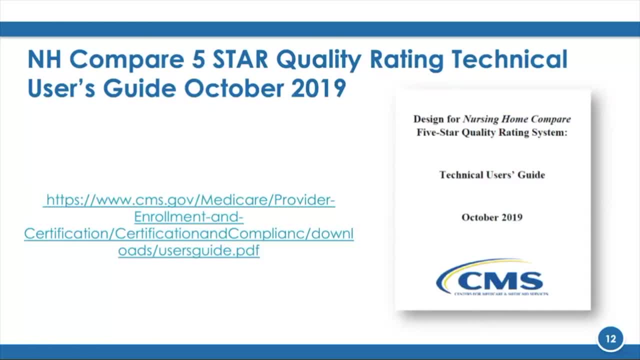 I know that I've provided you with a lot of information about the quality measure and score ranking. If you want to learn more in-depth information about this, you can find it in the October 2019 textbook. If you want to learn more in-depth information about this, you can find it in the October 2019 textbook. 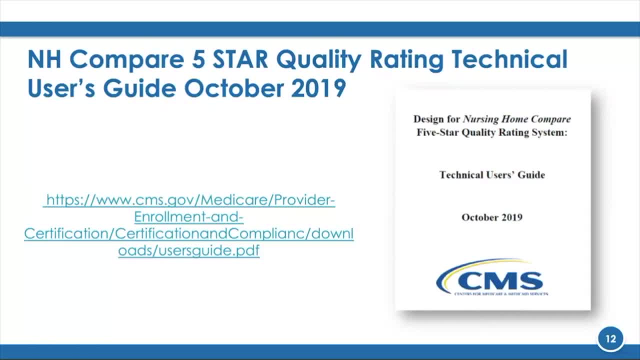 2019 Technical Uses Guide that I have referred to in prior slides. This guide is a good resource and will most likely address any questions you may have or will have to speak to about your measures, as it takes a deep dive into all of the domains. 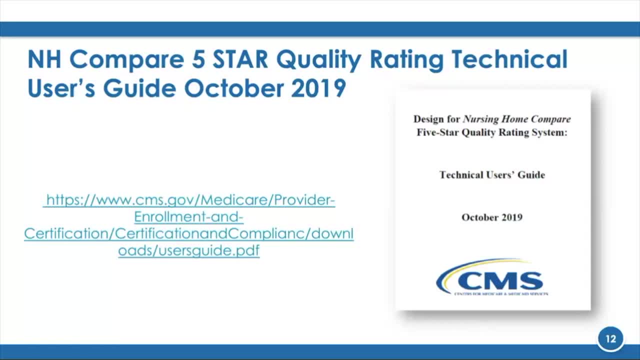 and how they factor in your star ratings. So here is the address or you can just search: CMS Technical Uses Guide- October 2019.. Make sure you specify October 2019, because there is an April 2019 version, but it does not have all of the current updates. 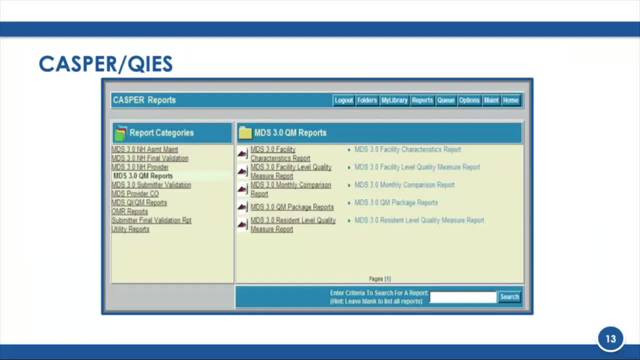 Next. So, knowing the significance of the quality measures in rating and overall performance, it would benefit the nursing homes to keep a close eye on these measures and scores, assessing improvements and implementing relevant interventions without having to wait for nursing home compare and the associated dated timeframes. 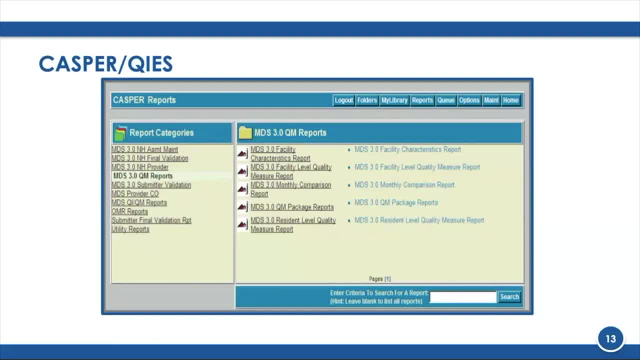 You may have a built-in electronic medical record and capability that provides you with QM data reports. but let's look at the information available to you in the CASPER Keys. So some of you may be asking: what is CASPER Keys, Certification and Survey Provider Enhanced Reports, or CASPER. 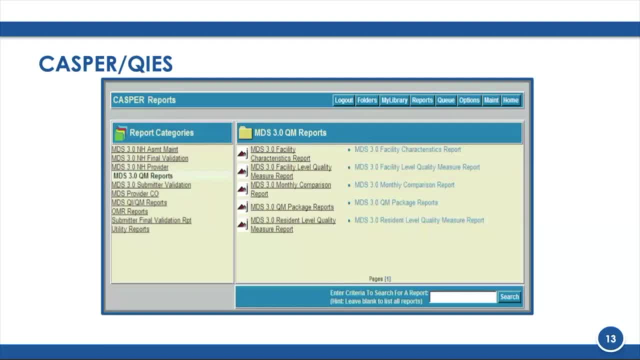 enables you to connect to the CMS National Reporting Database. CMS Healthcare Quality Improvement System, or QIES, is the source of the quality data. Through the QIES system, you will have access to CASPER Quality Measure Report page and its useful reports. 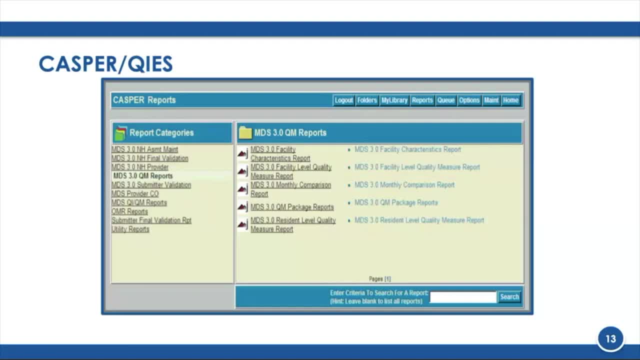 The CASPER QIES data is a resource for you to further assess improvement factors based on your quality data. The CASPER QIES data is a resource for you to further assess improvement factors based on more current data. Use of the CASPER QIES offers an opportunity to transfer data into improvement strategies. 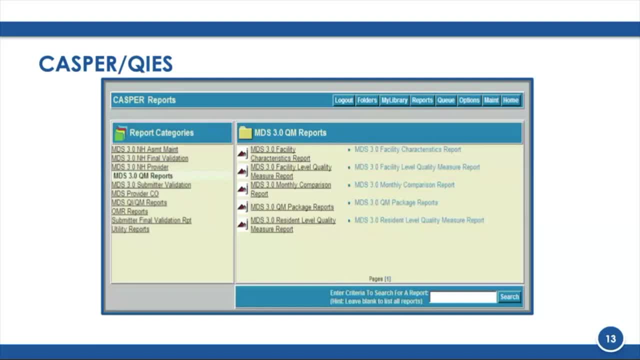 The CASPER QIES data are updated each Sunday with the data that was entered in the system within the prior week. You can review the direction the measures are going and further assess resident-level data to determine the residents that are triggering the quality measure. You can use the information available to you to determine the quality of the data. 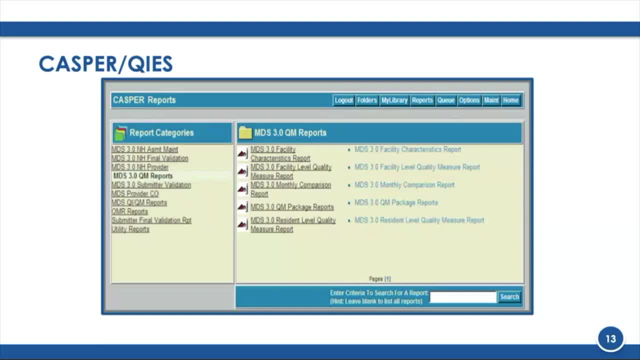 Use the information to target your interventions specific to noted problem areas, Reviewing the information on a weekly basis and working to make change in a way to make a measure improvements and to head off any negatives-nursing home- compare listing So, two reports that are available to you that I would like to discuss are: 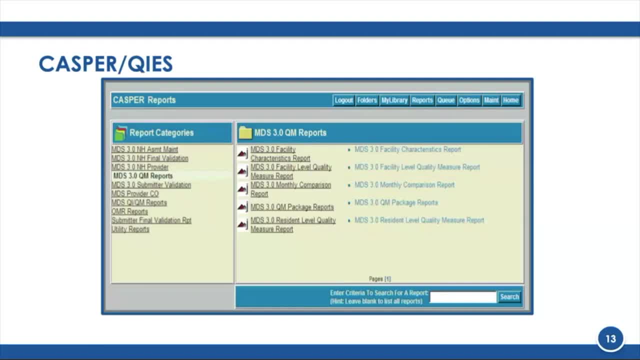 the facility level quality measure report and the resident level quality measure reporting. You can see them on this slide to the right in reports. Facility level reports list your facility's quality measures and rates and by looking at this weekly you can get a sense of how the quality measure rates are changing week. 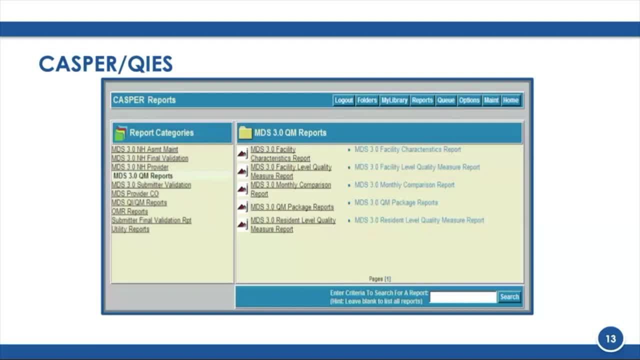 to week and you can assess the effectiveness of your improvement interventions. Next, look at the resident level information. It is here where you can see what residents are triggering the quality measure and it is here where you should be asking key questions. For example, why is the resident triggering the measure? 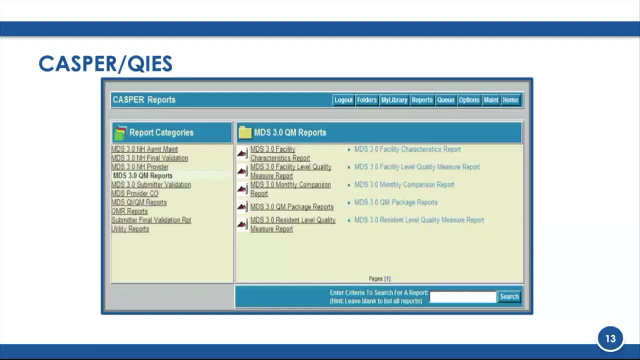 Is the information correct? Are most residents triggering the measures located on one unit or maybe have the same physician? How many measures are the residents triggering and why are they triggering multiple measures? You can see the questions will give you an idea of what the quality measure is and you. 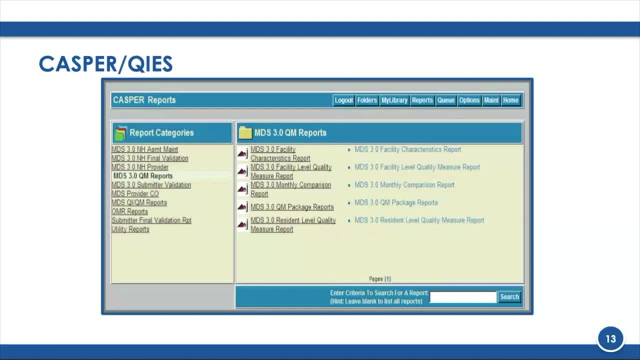 can review answers by looking at these reports. The information in these reports is useful for jump-starting quality improvement intervention. I bring the reports to your attention as additional and key review tools Knowing the QM rates, the residents that are impacting the rate, the individual QM point. 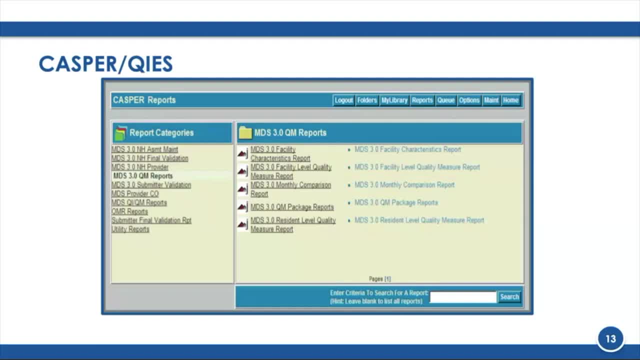 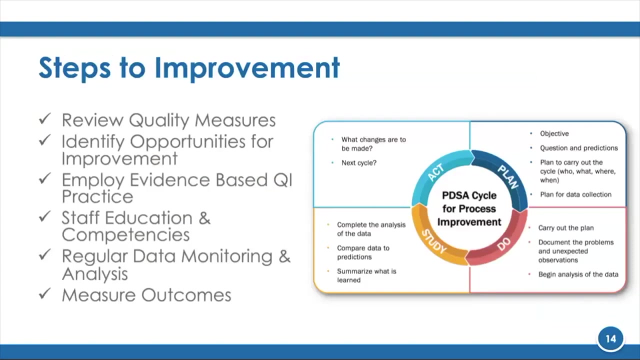 values linked to the total QM rating, are all important pieces of a quality improvement puzzle that can be used to direct your facility's performance improvement strategies and to measure progress. We drilled down and we linked the quality measures, their point values, star ratings. 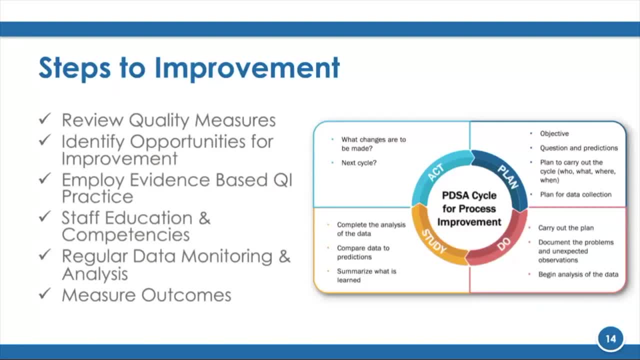 and how they factor in our quality improvement interventions. So the takeaway today is: bring it all home. When you get back to your facility, think about, or take a fresh look at, the quality measures and how they link to the measures of quality in your facility. 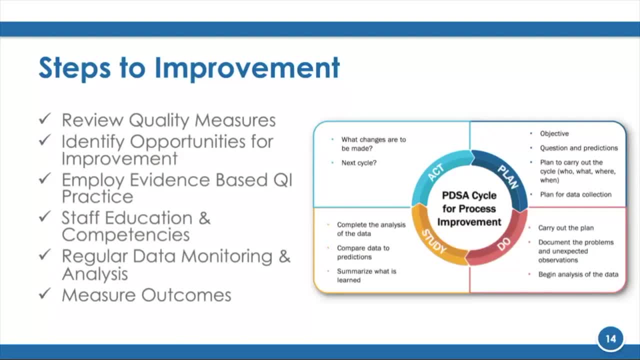 Begin by drilling down the QM information we discussed today and, as a team, dissect the information and see what it tells you. See what information you can gather to assess opportunities for improvement based on the information that is available to you, By prospectively understanding the QMs and how they drill down to assessing resident. 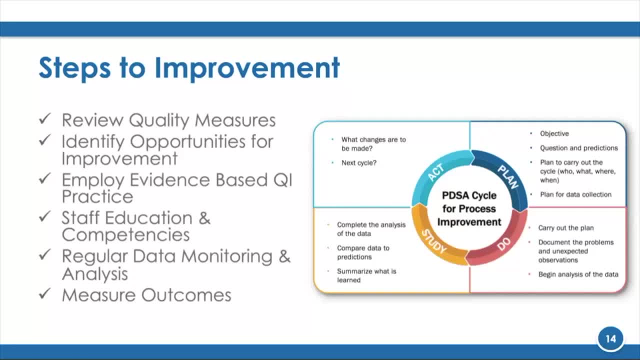 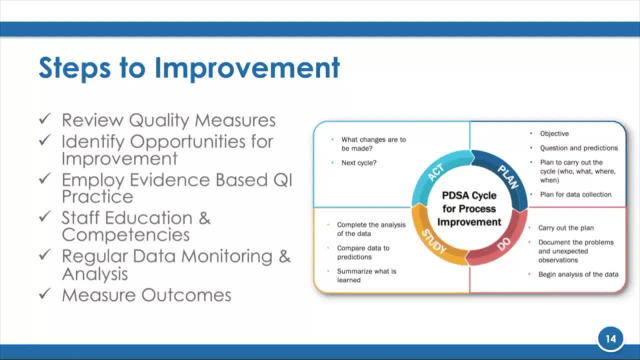 What QMs are in need of improvement to heighten the overall quality of your facility? What QMs are in need of improvement to heighten the overall quality of your facility lies in the low point threshold. You also note that many of the residents on Unit A 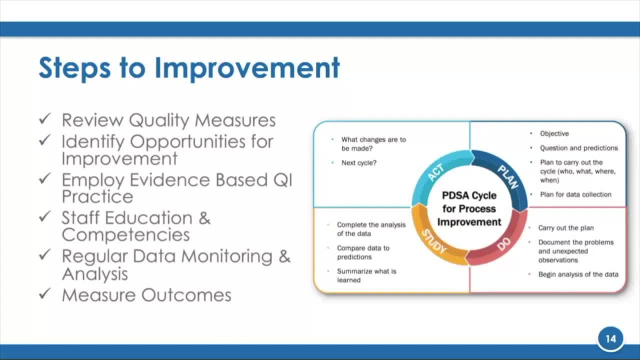 are triggering the QM. There appears to be a common denominator, as the issue appears to be on the same assignment with the same physician. So you can see, you now have a targeted opportunity for improvement and an area of focused intervention. In addition, we mentioned 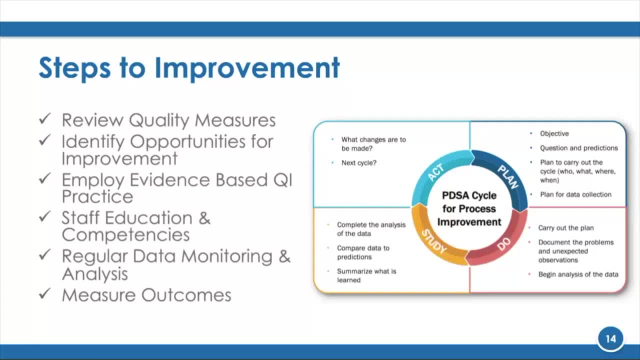 MDS and claims data that are the source of the QM rating. So it may be good to start to review and determine if the data is correct. Why have a negative outcome that is due to incorrect coding? Determine if staffs responsible for coding are kept abreast of current changes. 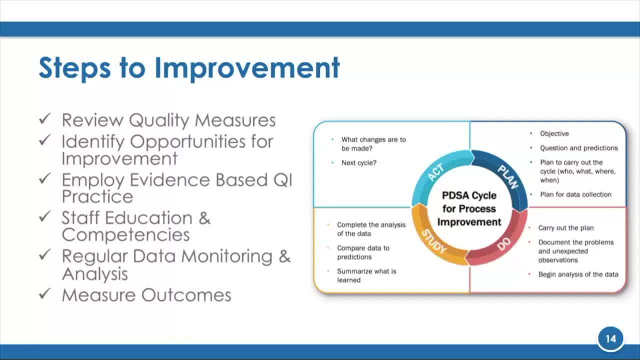 Is there an ongoing data audit review process? Are there areas that could benefit from additional education or competencies? Does the MDS and claims data include MDS and claims data that are the source of the QM rating? Does the data demonstrate identified opportunities for improvement? How can the data be transferred?